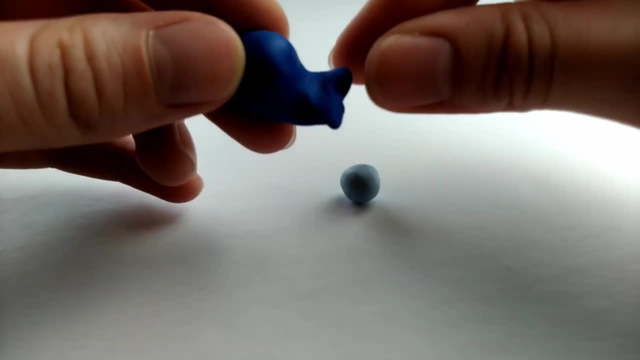 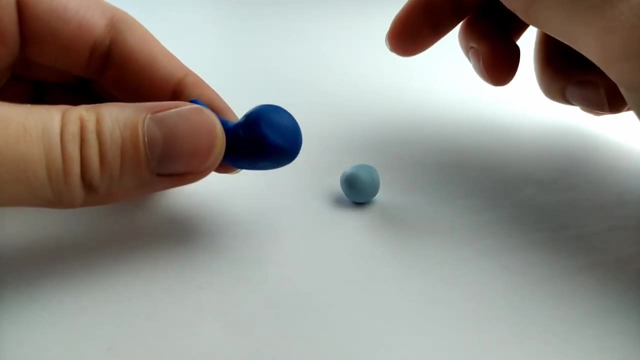 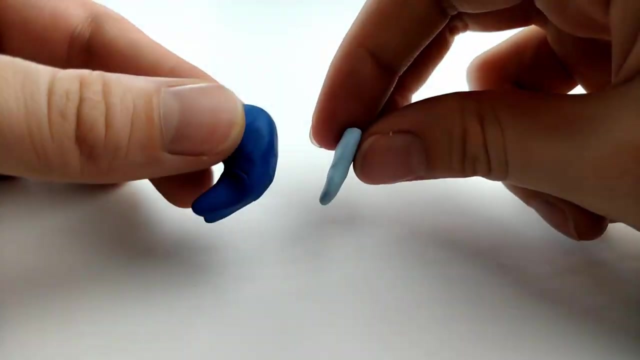 ballpoint tip or something similar, and split the end in two and pinch each side to create the tail. Now, with the smaller ball of the light blue clay, we're going to flatten it out into a teardrop shape and then press it along the bottom of the whale shape we created to create the underbelly. 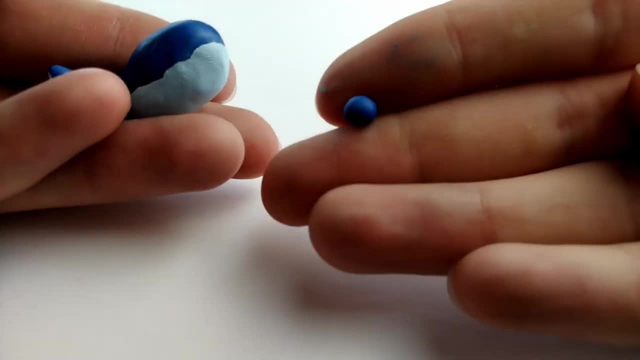 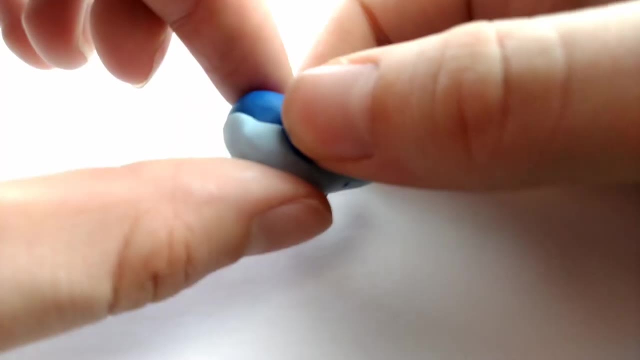 Once the edges are blended in, we're going to take two small pieces of the dark blue clay, roll them out and flatten them, And we'll use those for the flippers on the side. Now, you're just going to bake that in the oven. 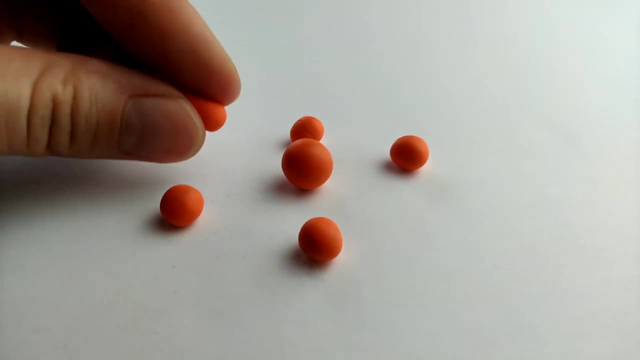 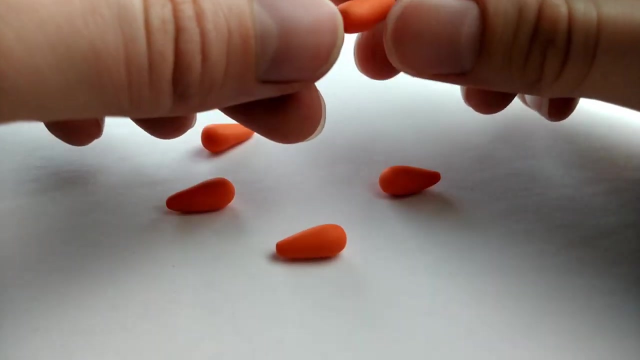 Next up is the starfish. Now we're going to start off with five equal pieces of orange clay and we're going to roll them into cones. Once that's done, we're going to attach each of the cones to a center piece of clay and we're going to smooth out the edges with a. 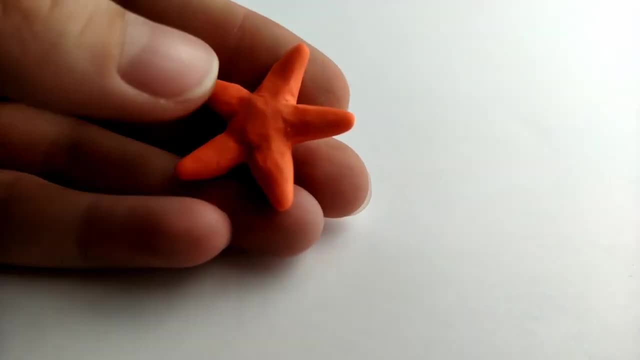 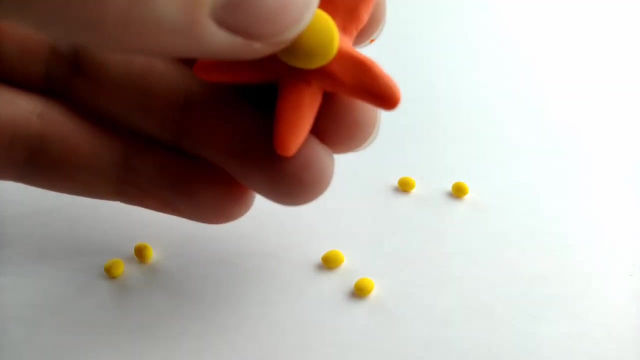 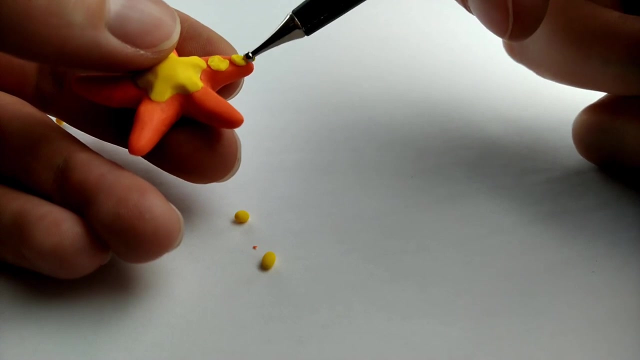 ballpoint tool. Once that's done, we're going to add a little bit of detail with small pieces of yellow clay, So just cover up the center and then use even smaller pieces and put two on each arm, And, after giving a little bit more shape to each of the arms, it's now ready to bake. 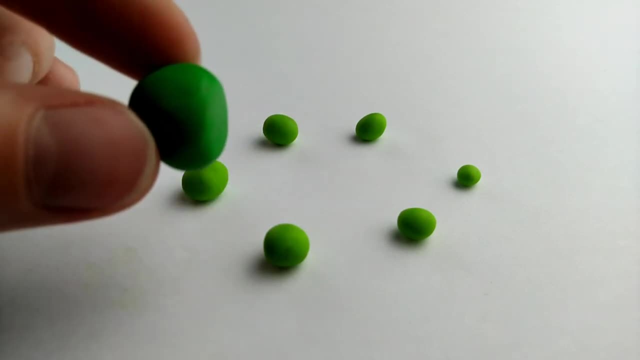 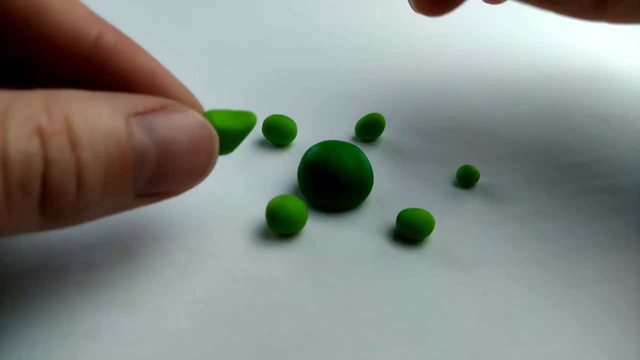 Next up, we're going to be making a sea turtle. We're going to start off with flattening one side of the shell against a table or your hand, Next shape the head by pinching the sides And, once you're happy with the shape, flatten out the end and place it underneath the shell. 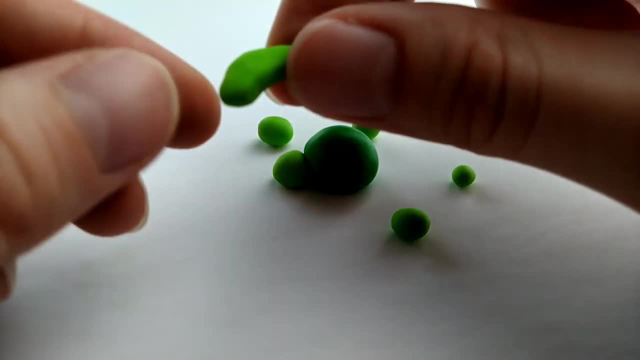 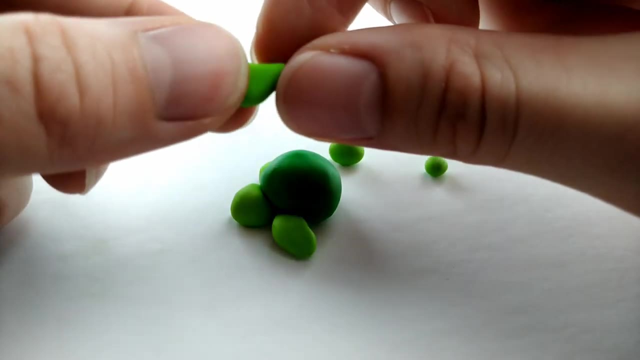 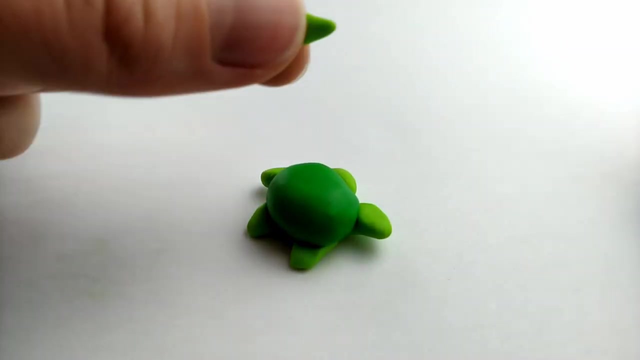 blending the edges together For the arms. we're going to pinch both ends of the ball and make it into a sort of triangle shape. Do that for both sides, and then make similar shaped legs for the back, And the last piece is just a small triangle for the tail. Now the only thing left to do is take a 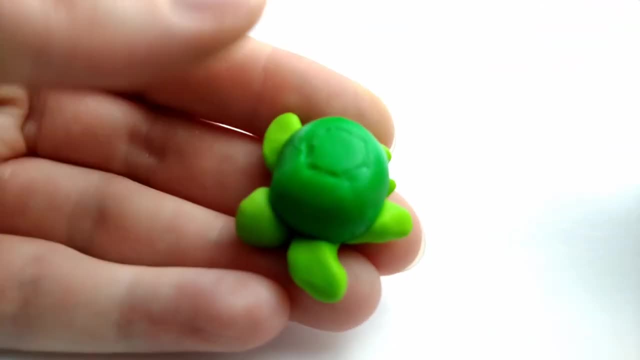 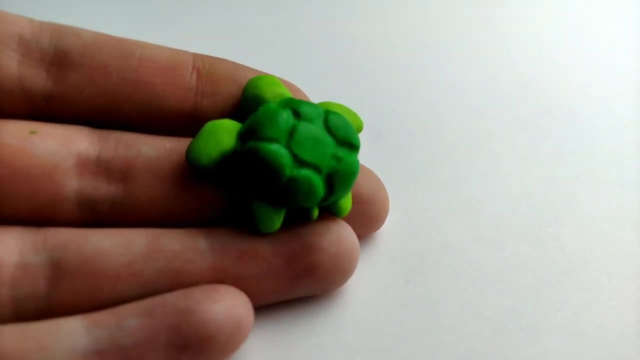 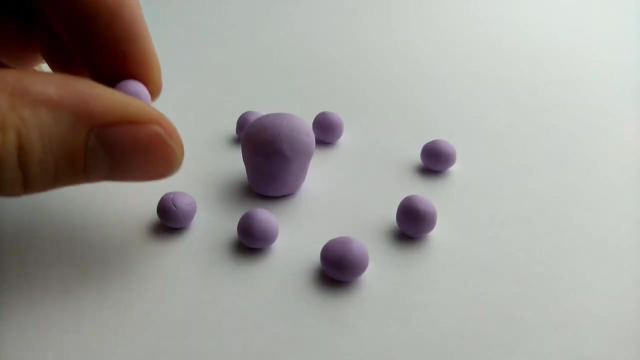 cutting tool or a toothpick and draw out the shell design For this one. we'll be making an octopus. So start off with a ball of light purple clay and pinch the ends to extend the body. Take a smaller ball of clay and roll it out into a cone. 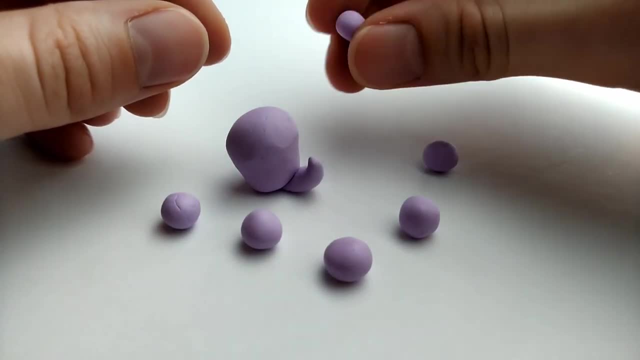 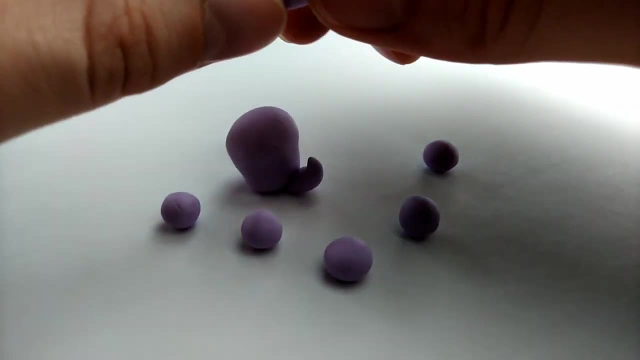 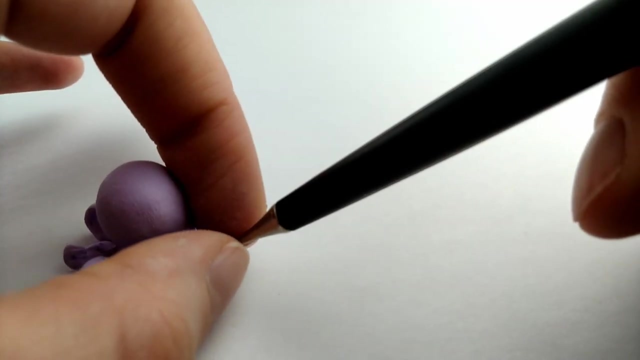 with a pointed tip and then curl the tip over. Do that seven more times to create eight tentacles. attach each of them to the bottom of the octopus And once all of your tentacles are attached, we're going to take little tiny pieces of dark purple. 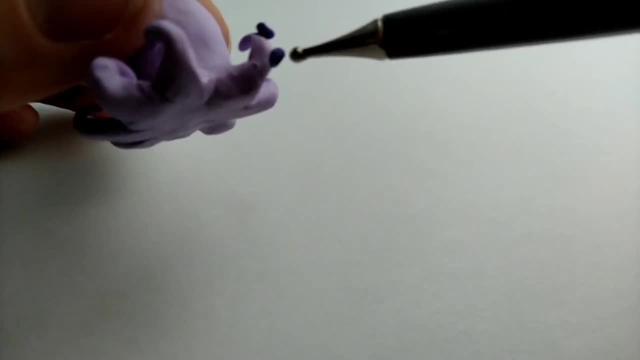 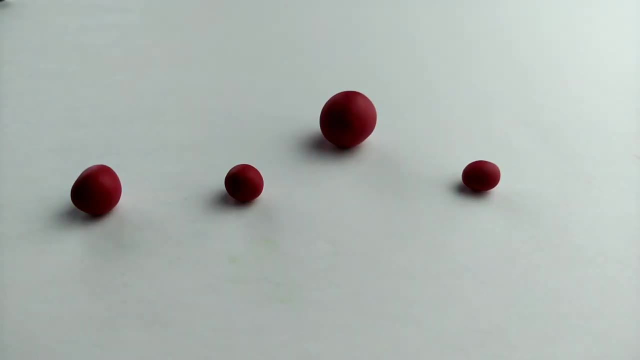 clay and roll them into balls, then press them into each tentacle to create little suction cups, And this one's ready to bake. Finally, we have a little crab to make, so start off with a ball of red clay. So we're just going to flatten off the bottom of the body first, And then we're going to 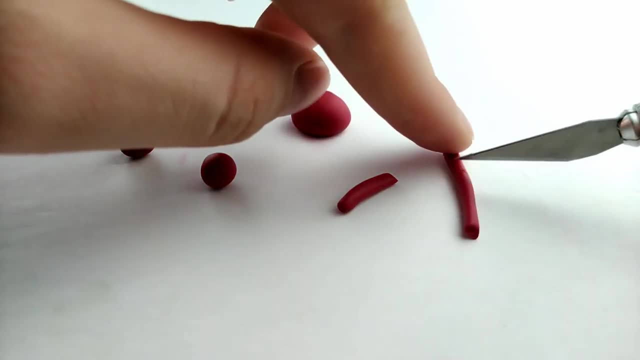 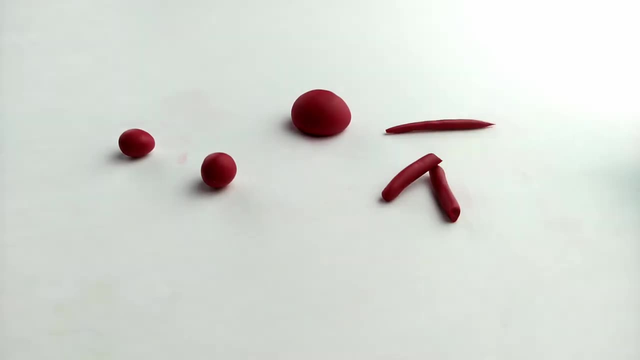 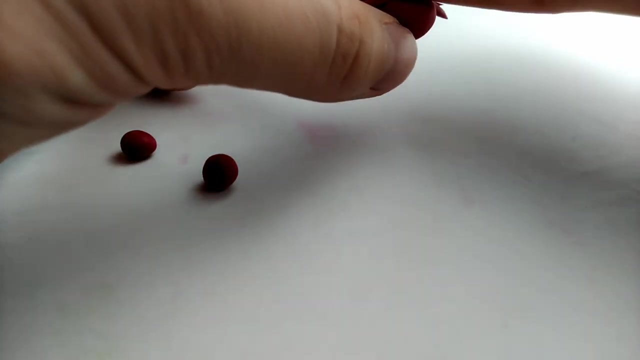 go on to the legs. Roll out a piece of clay and then cut it into thirds and then take each third and roll out each end into a point. Then you can take each leg and place it in the center of the bottom of the crab so each end sticks out. Now for the arm. take a ball and split it in half. 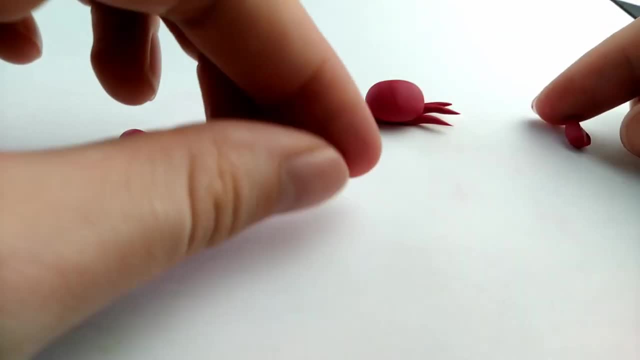 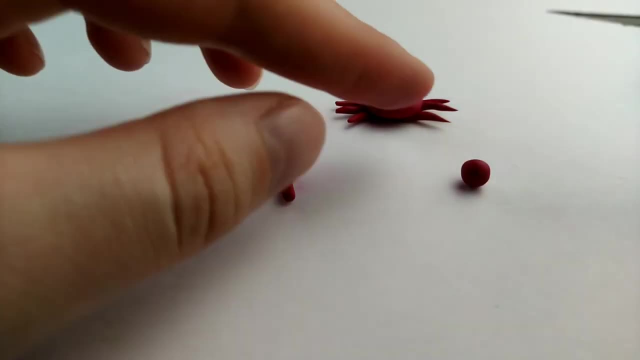 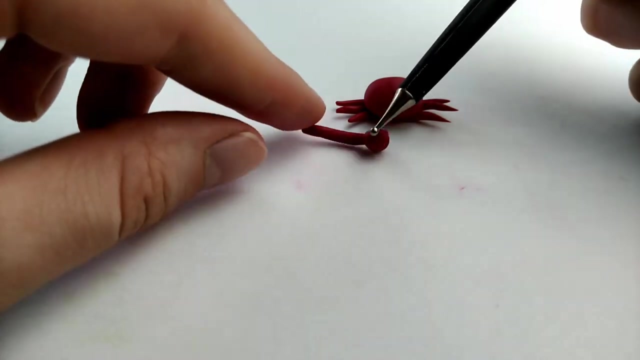 Roll out a log for one half and roll out a ball for the other half, And we're going to use that to shape it. Cut out a shape and connect them together to create the claw. Now you just gotta position the arms where you want. Cut off any excess. 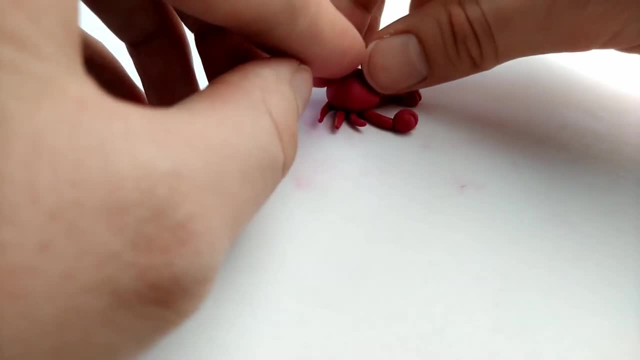 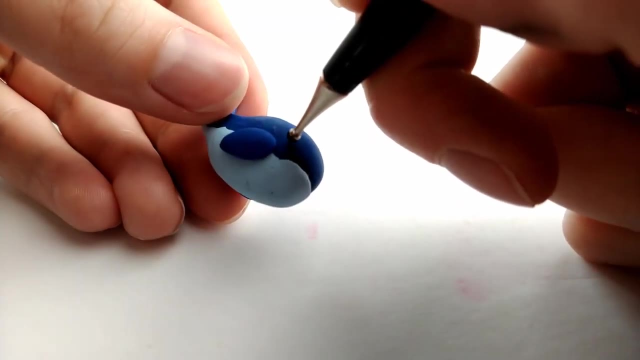 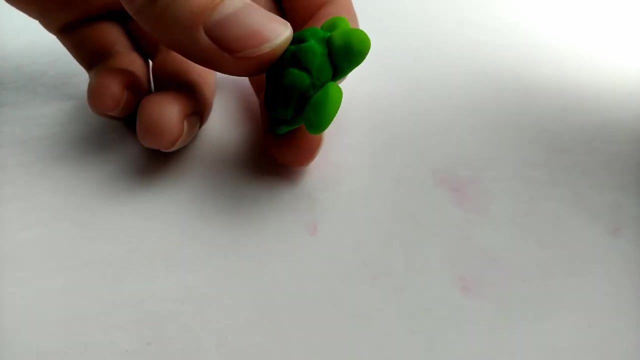 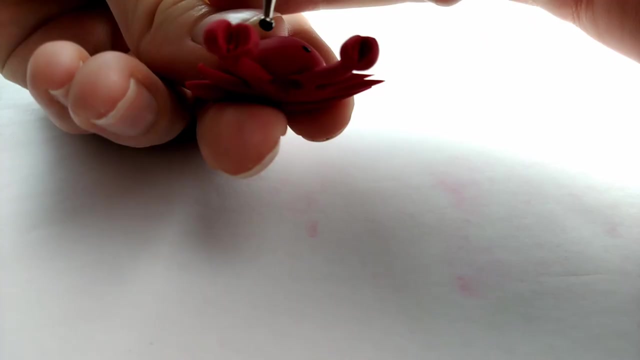 and then place the crab on top and blend the pieces together. Once everything is baked, all that's left to do is to add a little bits of details. So I just added some eyes to some of my creatures. And there you have it: Five easy sea creatures. Let me know which one is your favorite, or if you. 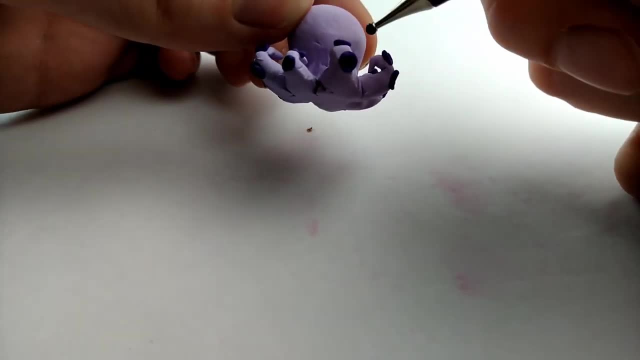 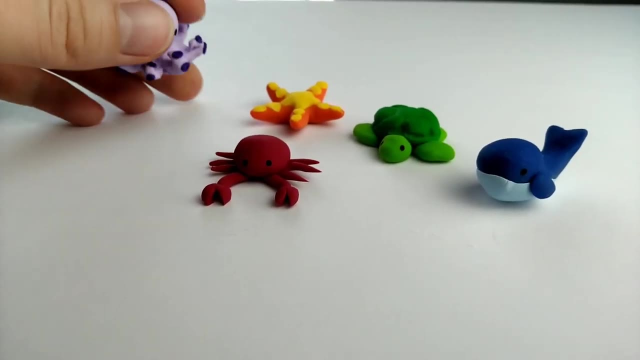 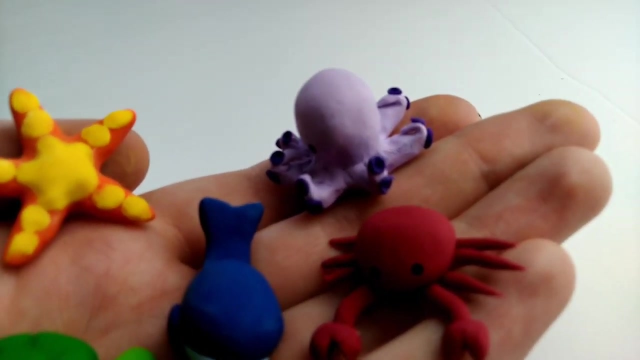 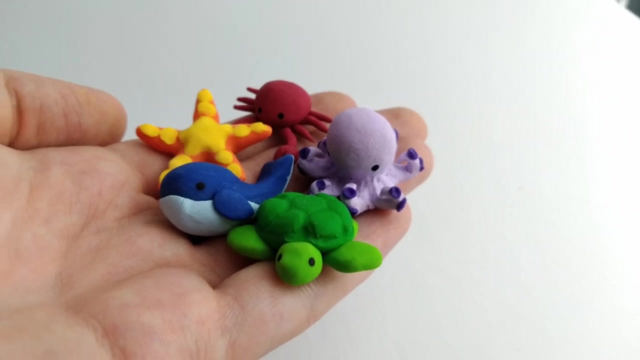 have any suggestions on what you want to see next? just leave a comment down below and I'll be sure to look at them And I'll see you in the next video. Bye. Other than that, hope you have a great rest of your day and I'll see you guys later. Bye.